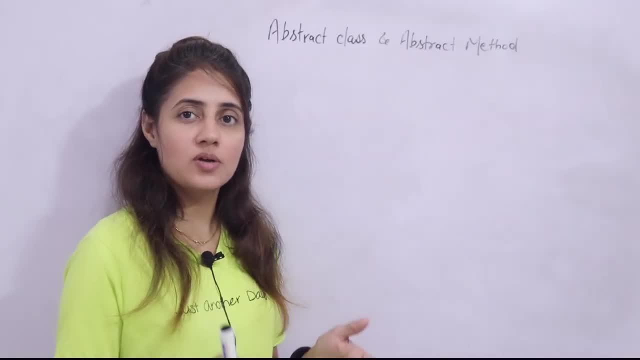 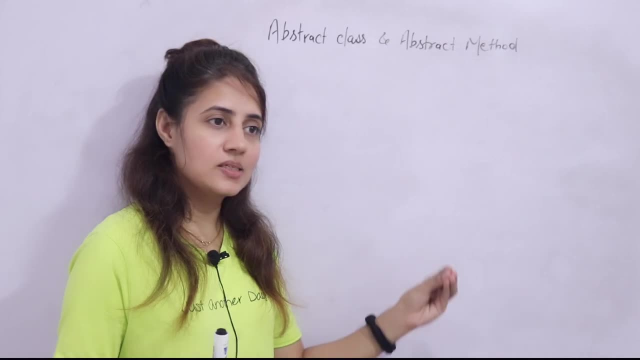 Hey everyone. I hope you all are safe and doing good. So in the series of learning Python programming language in the previous video we have seen what is abstraction. right Now in this video we'll be discussing about abstract classes and abstract method. Basically, we'll discuss 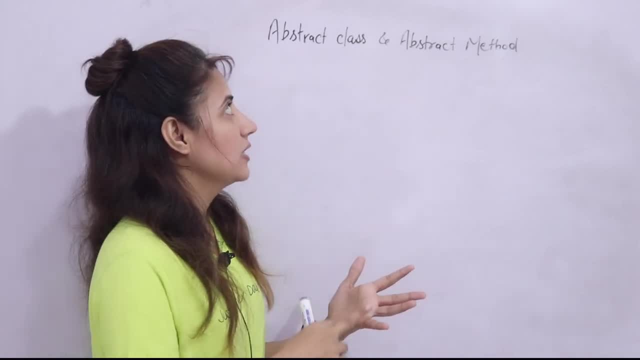 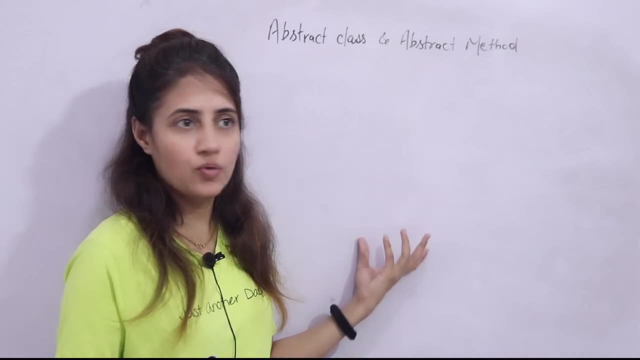 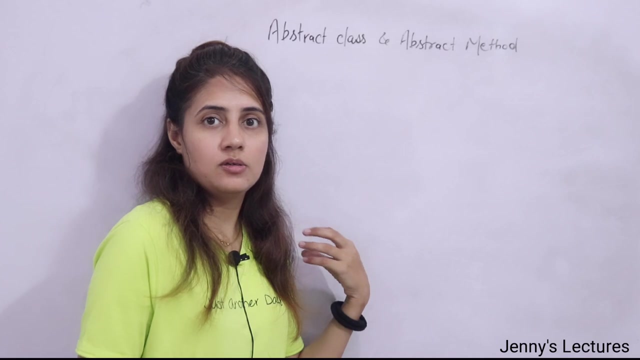 answer of two questions like what are abstract classes and what are abstract methods, and why we need these things, Why we need abstract class, Why we need abstract methods, Why we make our classes abstract classes and why we create our. you know why we create abstract methods in those. 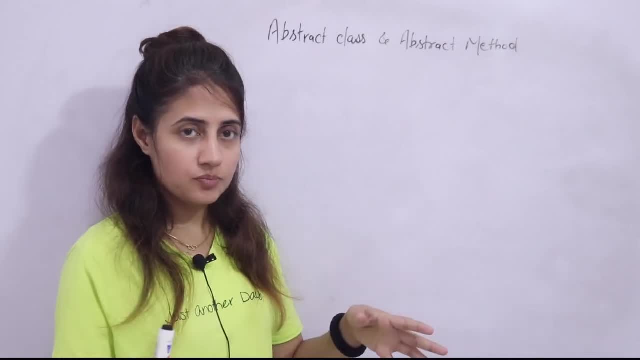 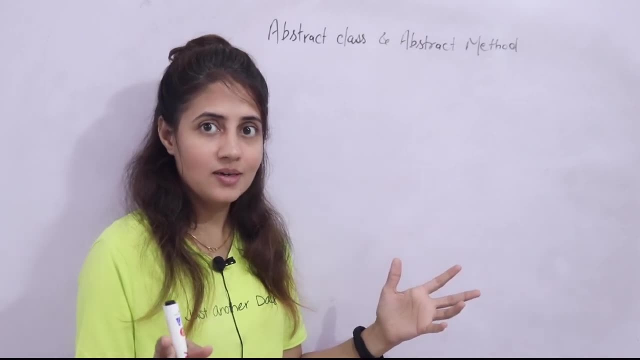 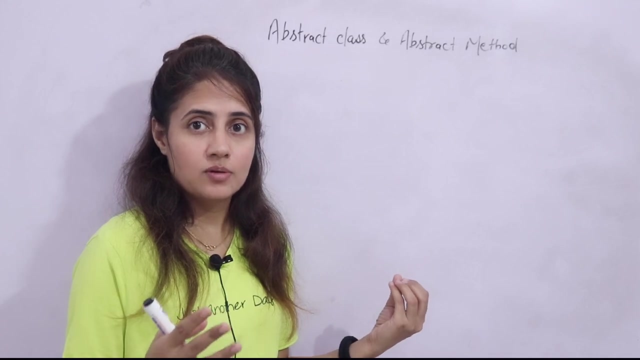 classes, right, These things we'll be discussing in this video. Now let me just first tell you one thing: Python by default doesn't support abstraction, right, Like we have like in C++ and Java. So but yeah, we can implement or we can achieve abstraction in Python, but because we 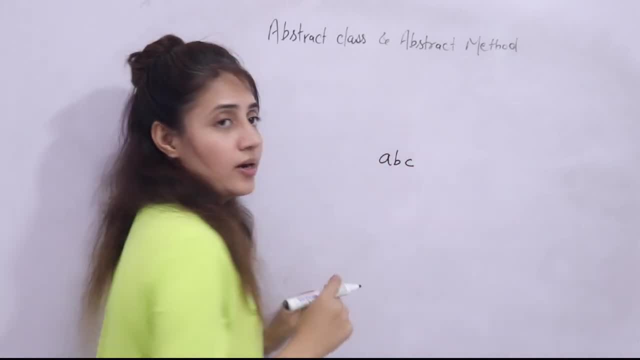 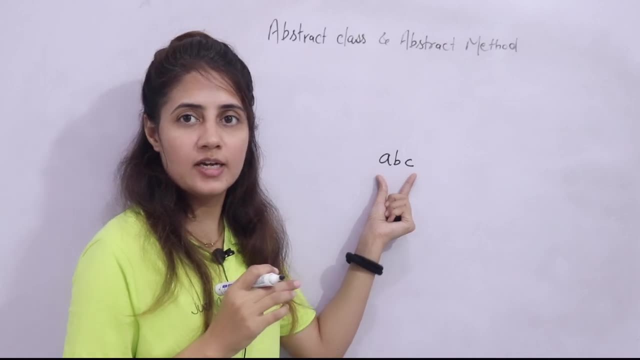 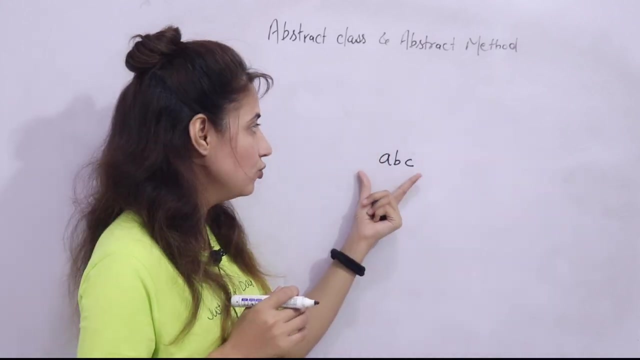 have a module- ABC- Abstract base classes, ABC- abstract base classes. This module we have and using this module we can achieve abstraction, We can make our classes abstract classes and we can make method abstract method. right, So you have to import this module or you can say: from this module. 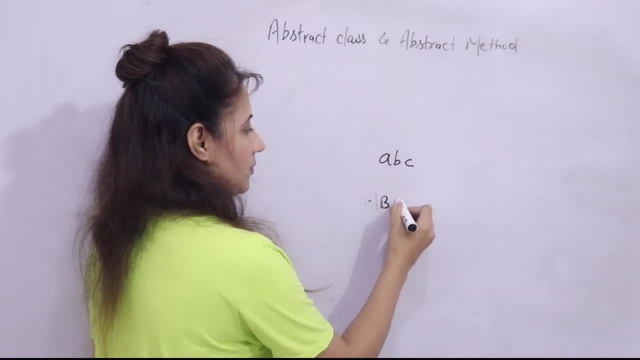 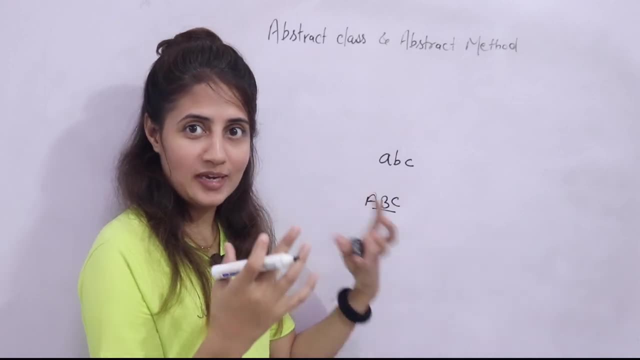 you have to import ABC class, ABC class right Now, how you are going to create, how you are going to make abstract classes, How you are going to make subtract or subtract method. Let's see practically Okay. So this: 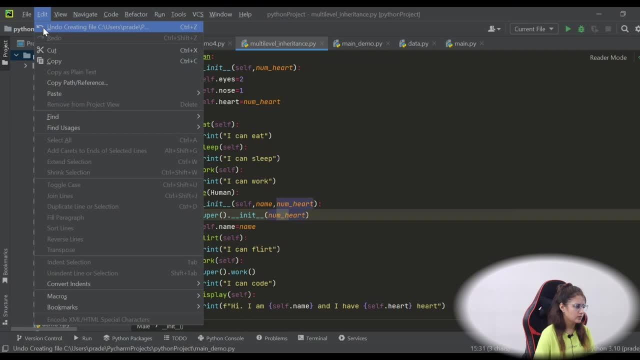 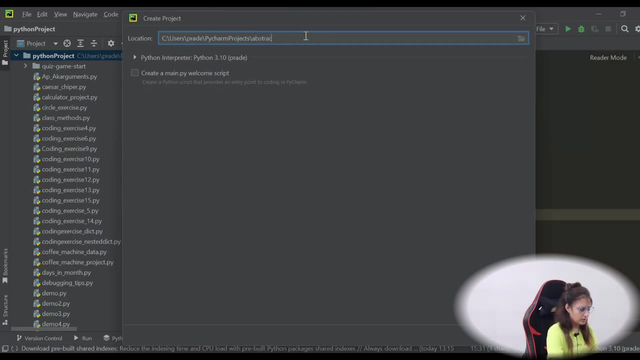 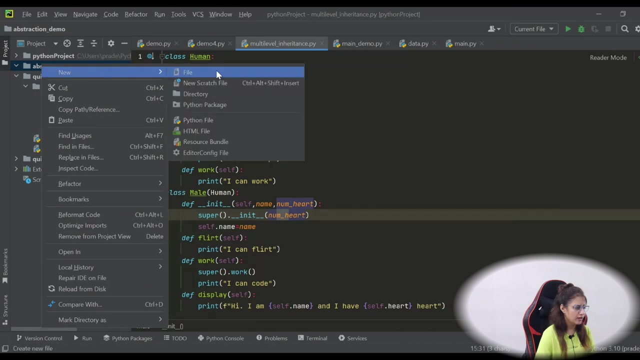 time I am going to create a new project, right, So click on file the new project. and the project name is abstraction underscore demo. right, So this project. we have abstraction demo. Now right click on this project and create a new project. So right now, I am going to create a new project. 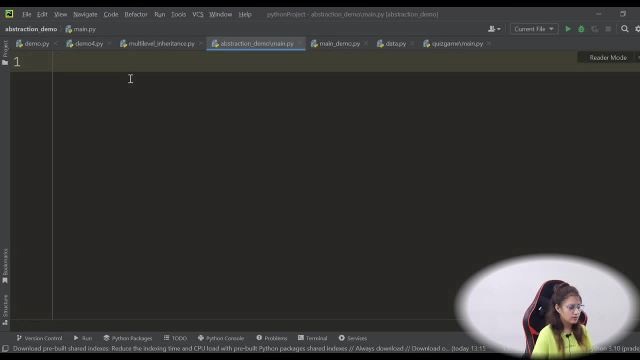 file: main dot py. okay, so first we'll see what is abstract class. let's take first a simple class, normal class example. we have a class. suppose we have a class like bike, right, and in this bike obviously we are having some method like bike will start, stop like this. so i have a method. 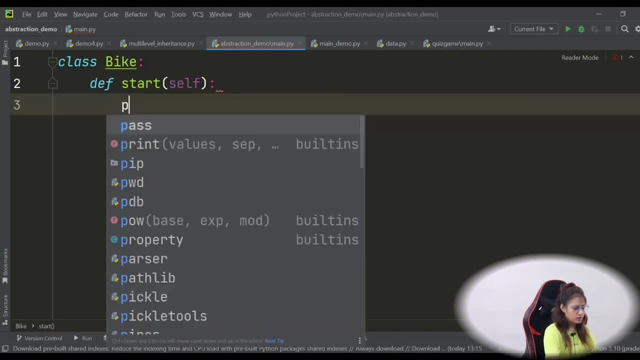 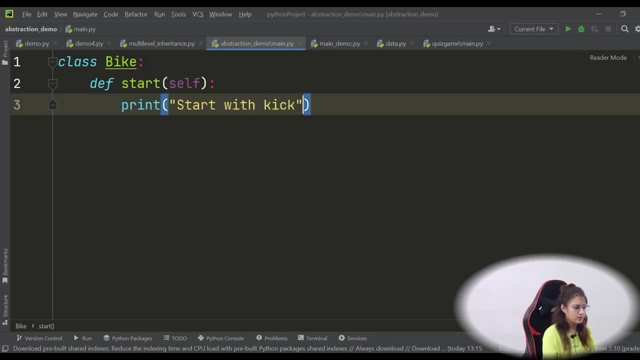 start right and just here print: start with cake. okay, now suppose i have another class. we have a class like scooty, so this will also have a method start. i'm having self start, scooty self start, and suppose one more class. let's have one more class and 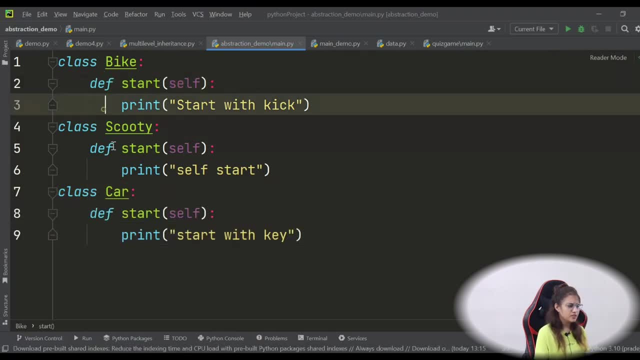 that is like car. so three classes we have and same method. they are having start, start, start. but implementation of these method are different. for bike it start with kick, for scooty, self start. for car it start with key right and obviously they are having some attribute, also like number. 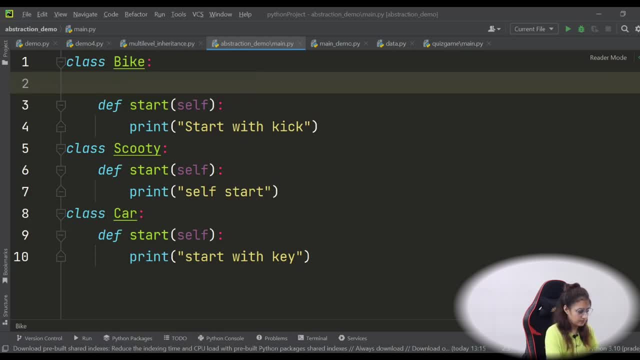 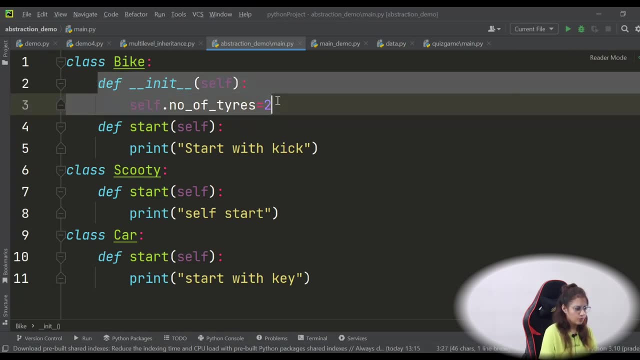 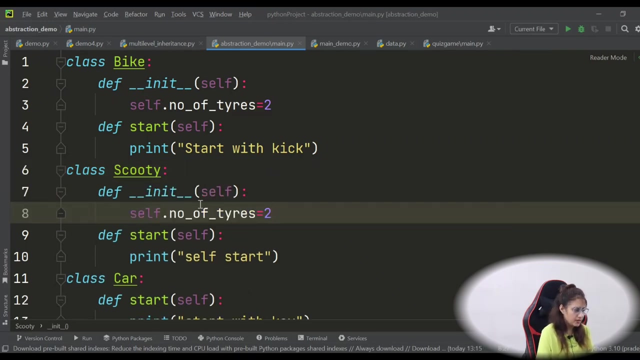 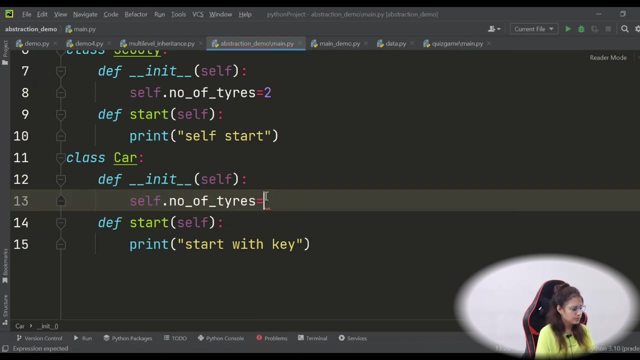 of tires so we can have a constructor. number of tires is equal to in bike we are having two tires. so in scooty also we have some attributes, so they are constructor like in it and we initialize these number of tires in scooty also to in car also we have like number of tires in car we have. 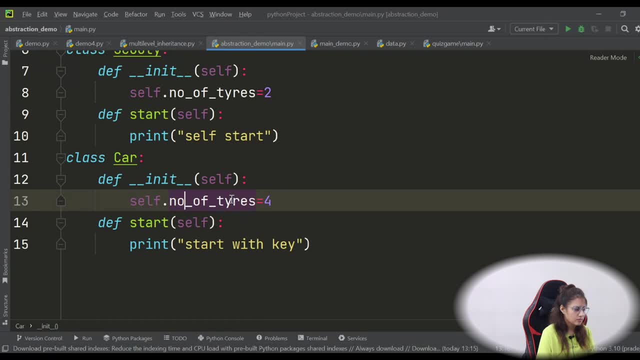 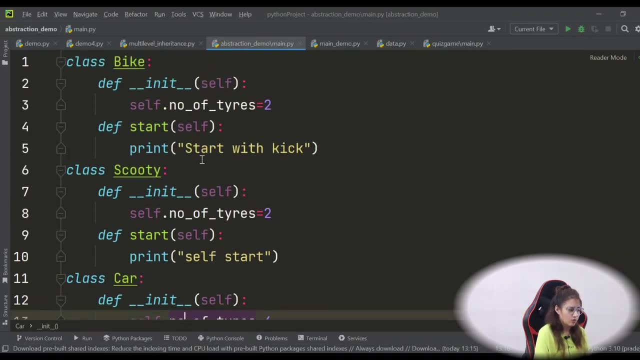 four: right: one attribute is this: now, every class, or there can be much more classes of this type, like truck or many other classes like this. so we have some attributes, so we have classes. also, right, and everyone is having same method: start, start and some number of tires and 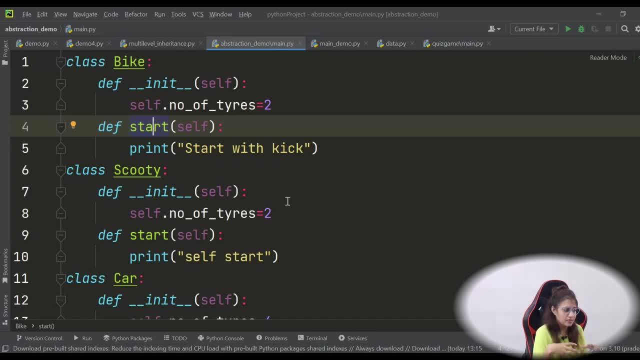 all this kind of thing, same same things every class is having, or the object of every class. right, actual bike is what object? actual scooty you drive is an object. actual car you drive is an object. so it's just a class, but actual object they are having similar kind of property. 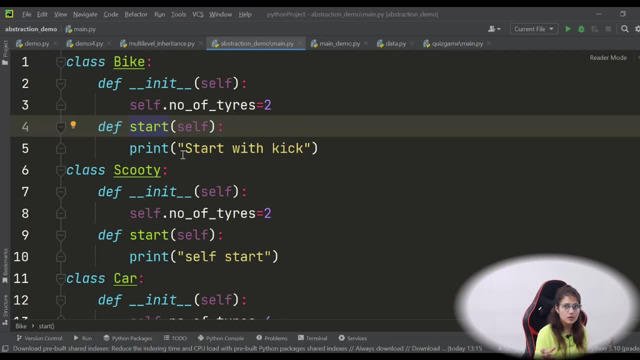 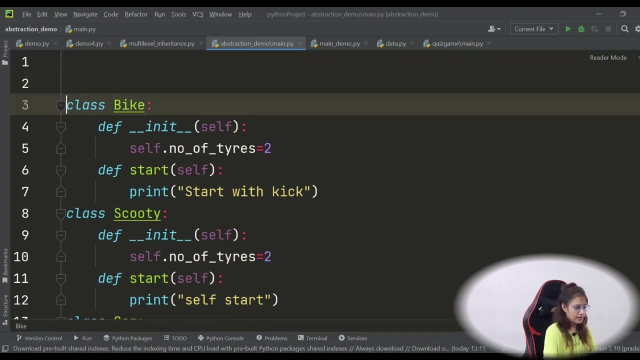 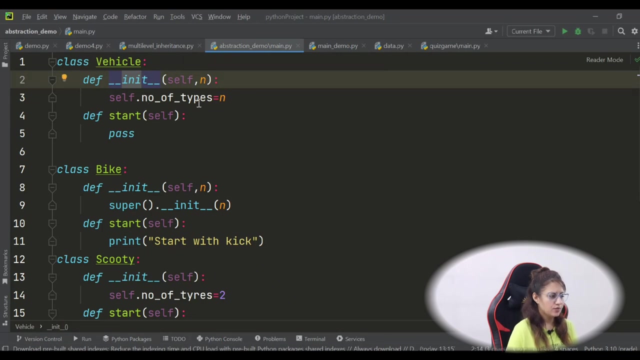 like. actually, each technique includes learning following each terms also, like you can say, such as above class, also usingрем, Allow, respect a class, product not using, and this will statistics, as you know, if we have haveificating these categories, or you can say methods or attributes, right, so what we can see here. we can make a blueprint of these classes, like a vehicle class. 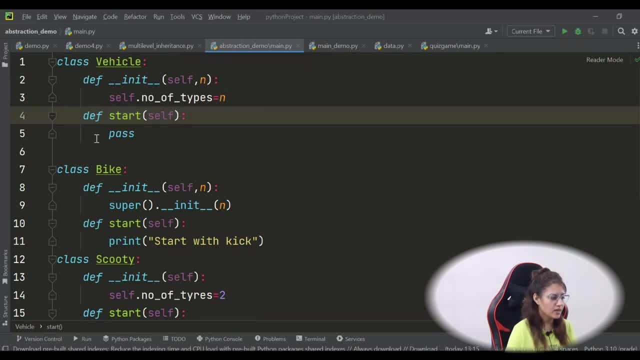 and one method, that is start, and in start it's empty. we are not passing anything like how the vehicle is going to be start because vehicle is a generic term. right vehicle can be like what it's: a car, scooty, bike, truck, anything- and they. 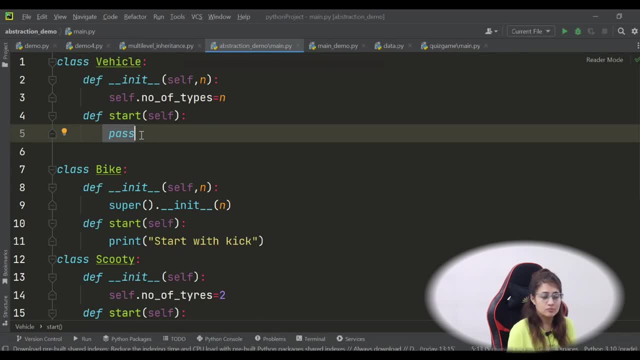 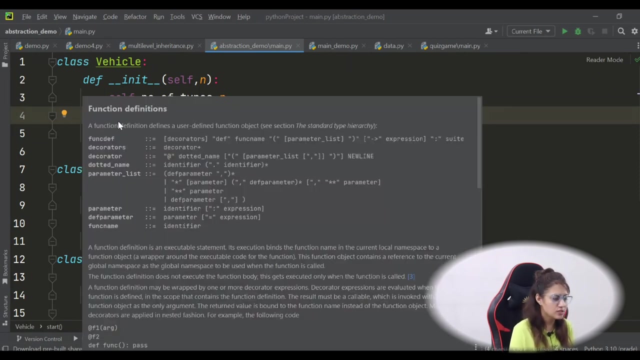 are going to start. you know they have their own method: self start, start with key start with kick and all right. so vehicle is a generic class. we can't define this start method means we haven't defined this start method here. we haven't implemented this start method here. we have just declared this method. 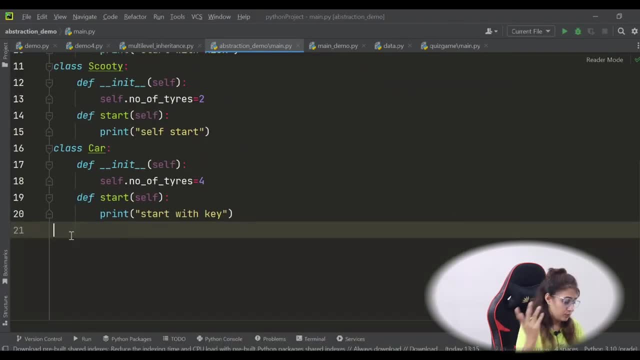 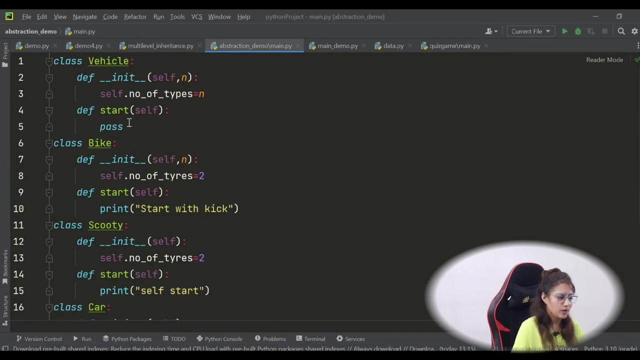 here. okay now, if let's suppose create a object of vehicle, class V is equal to vehicle and we don't know the type of vehicles. so how many tyre you will pass here? and if, using object, you want to call start, then obviously in start we are not having any implementation. so what is the use of creating? 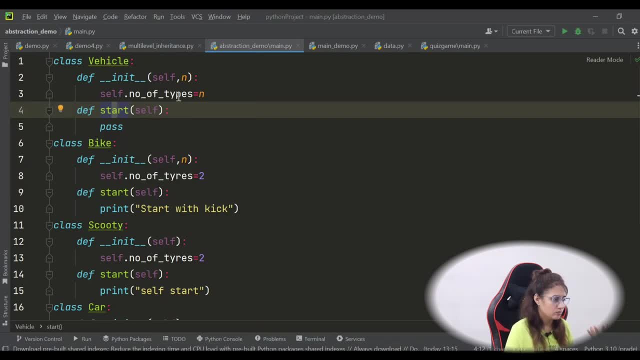 object of this vehicle class and calling start method and obviously we don't know number of tires to be passed right. so it's better to not create object of vehicle class because it is generic class. object is specific, like a bike. actual bike is an object. actual car is an object. 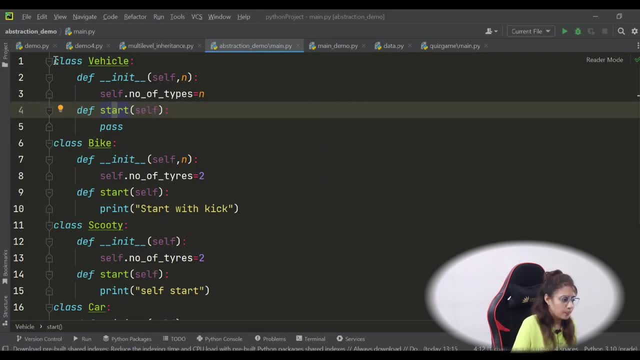 actual scooter is an object, right? so we want to restrict ourself from creating like object of this vehicle class, or we want to restrict anyone who is working on this project. maybe it's a big project, right, it's an application. or we are working on a software like this, right, so you? 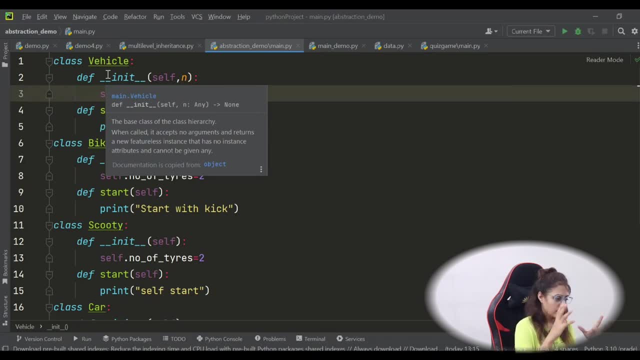 want to restrict someone or any, anyone, any programmer or any developer who is using your code or this class to restrict them from creating object of this vehicle class. right, so we want to restrict ourselves from creating, creating, you know, object of a particular class. then make that class abstract class. it's like a. 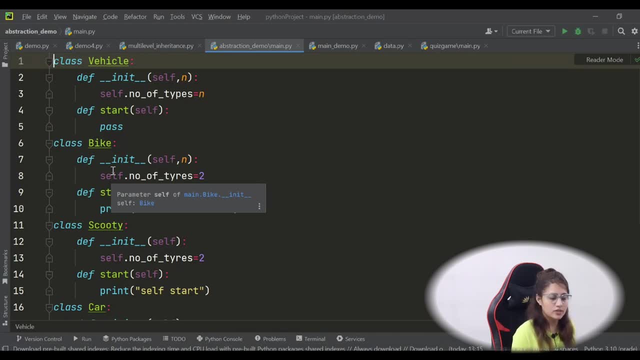 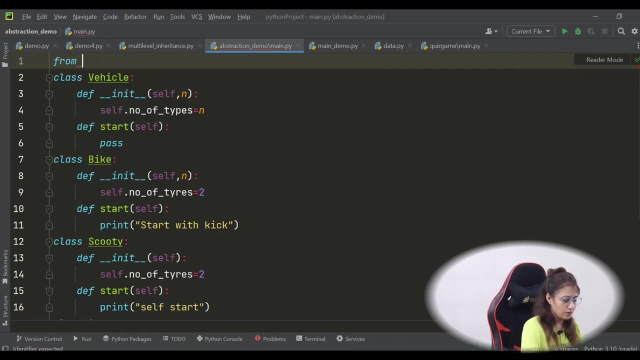 blueprint for all the classes. it's like an interface or it's like some set of rules, right? so how to make this class abstract class? first of all, you have to import, like from abc module. we will import abc class- sorry, abc class right, abc class- abc metadata, like after 3.4 version in: 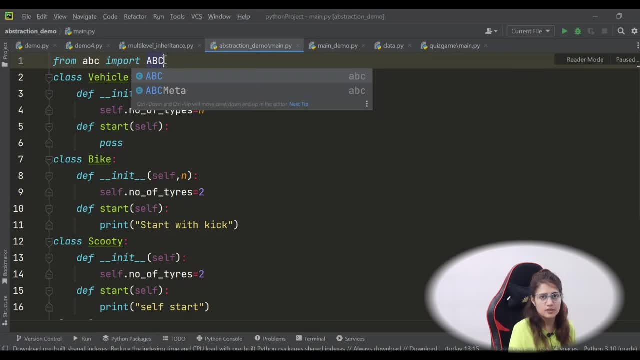 python. this is the new syntax, import just abc. but before 3.4 we were supposed to import abc metadata and that was different syntax, right. but now just import abc, right. and which class you want to make abstract vehicle class. so just inherit this class from see abc. this is a class c. here is c in blue circle c. so this is a class from abc module right. 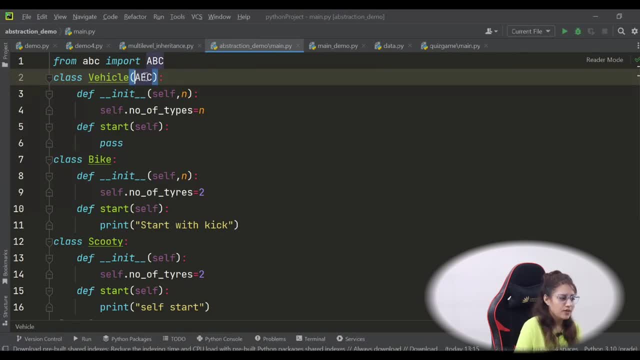 so now this vehicle class we are importing from abc, but it's not still now abstract class, because, and for a class to be an abstract class, it should have at least one abstract method. but we don't have any abstract method. yeah, yeah, yeah, yeah know abstract method. basically, let me just tell you: abstract methods are having only declaration. 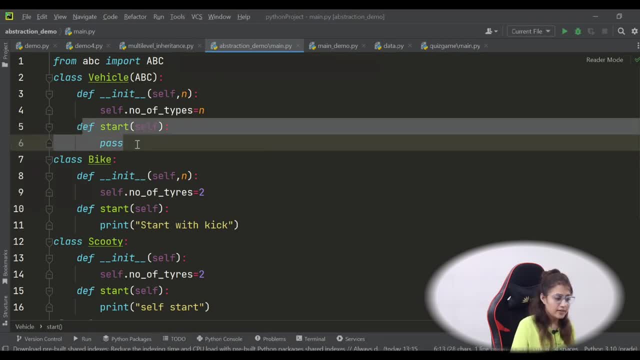 no definition. so maybe you will think this method is having only declaration, no definition. so this is abstract method. but no, in python by default this method is not considered as abstract method. you have to make it abstract using some decorator, right, and decorator is abstract method. so for that. 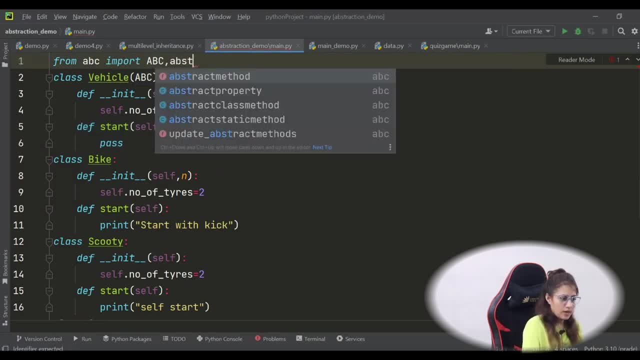 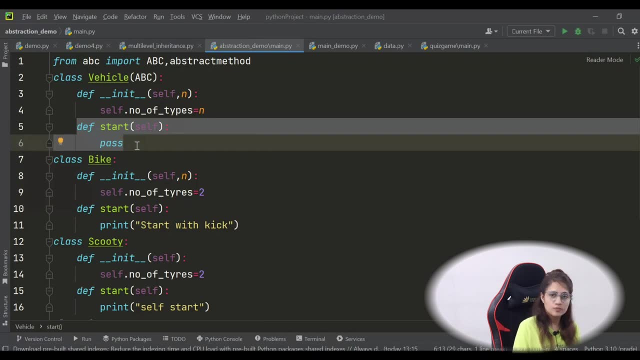 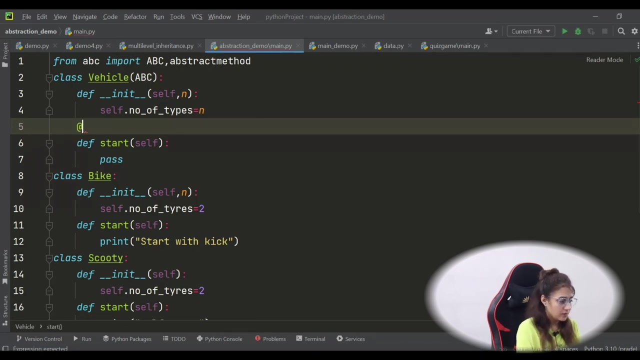 also, you have to import from abc module abstract method. this thing, right, and this method you want. you want to make this method abstract method. so before starting this method, you have to use a decorator. that is abstract method. add the rate and this abstract method. this, now this method, is abstract method. 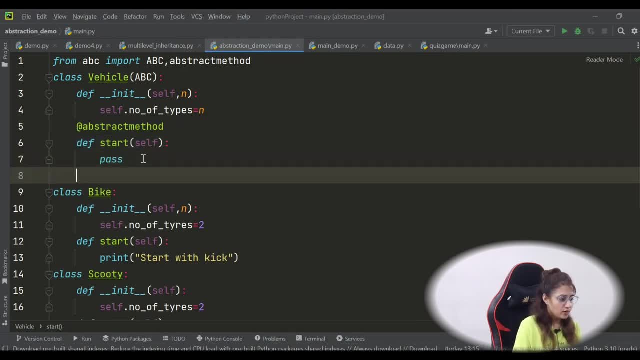 right. so now we are, we cannot create like object of this vehicle class right, so we can separate out our code. we are just, you know, using a small example. that is why everything i've written in the same code. but if you are working on a large project, just separate out your code like this: 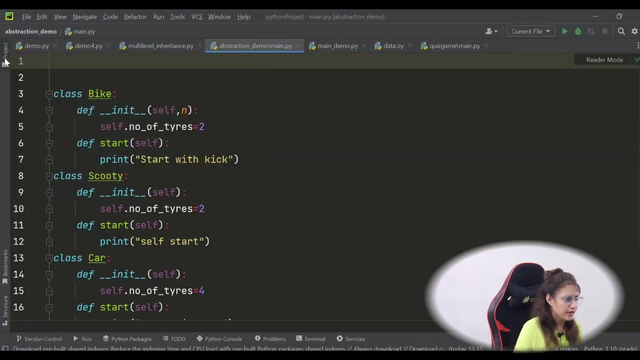 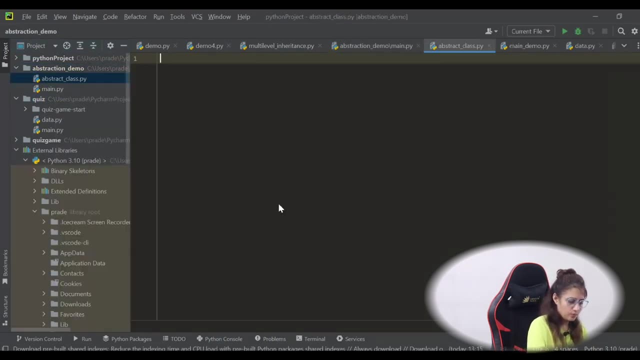 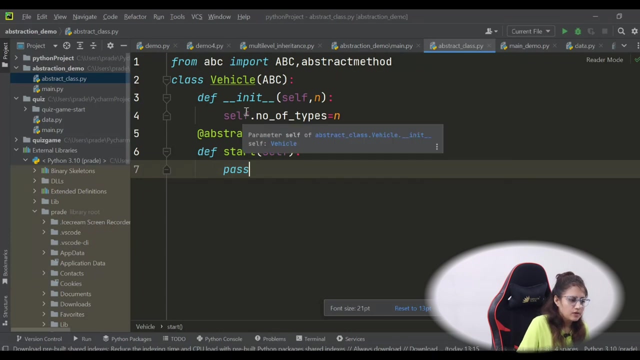 thing: this my abstract class i'm going to create in a new file. okay, so in my project abstraction demo, let's create a new file and dot v1, right? so here i'm going to create this abstract class, right? maybe you think like, if you do not, you will see here now. 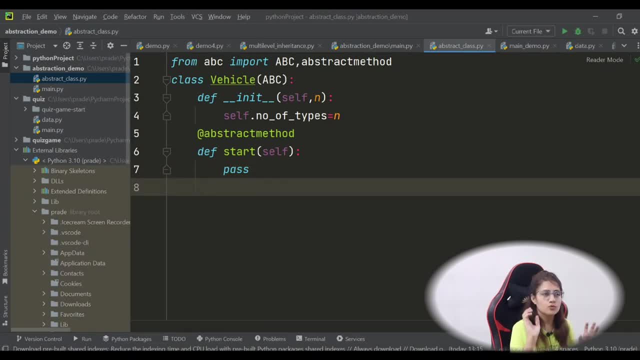 now, abstract class is what which is having at least one or more abstract method. it can have many more abstract method, one, two, three, four, but at least it should have one. if there is no abstract method, then that is not an abstract class right, and we cannot instantiate abstract class. it means what we cannot create: object of abstract. 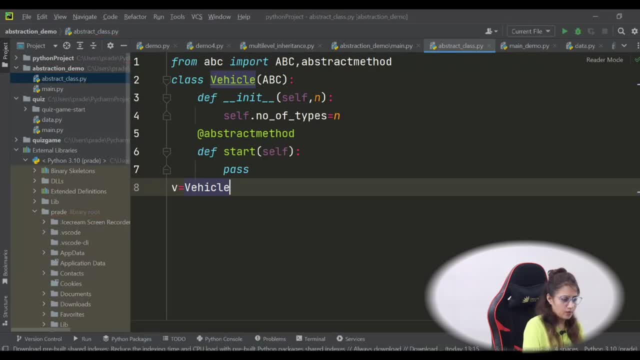 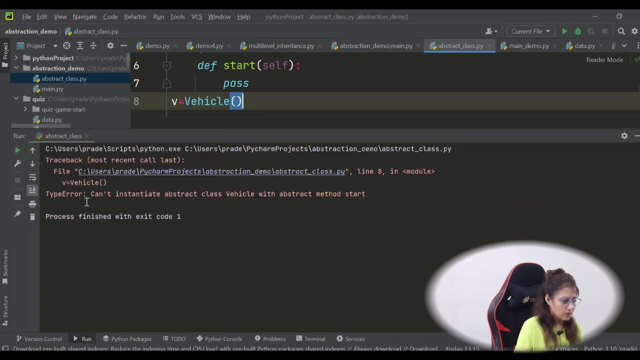 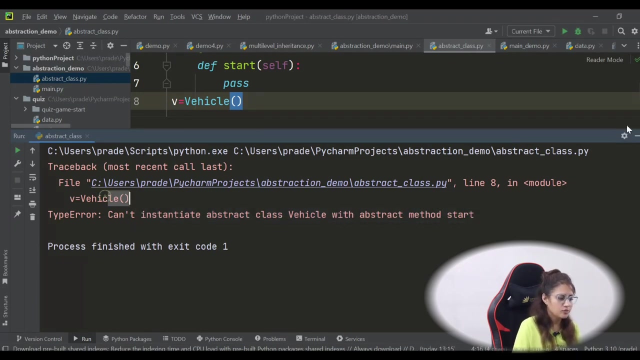 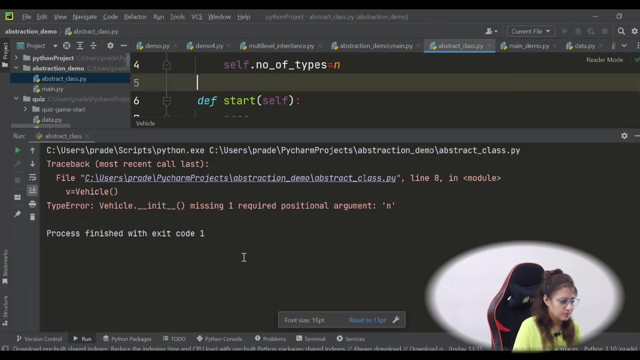 class. suppose you want to create object. v is equal to vehicle. i want to create object of this class, right, let's run this. see, cannot instantiate abstract class vehicle with abstract method. start. we cannot create object of an abstract class, right? but if you remove this decorator, if let's run this now, you can create object, but it will give another, you know. you can say: 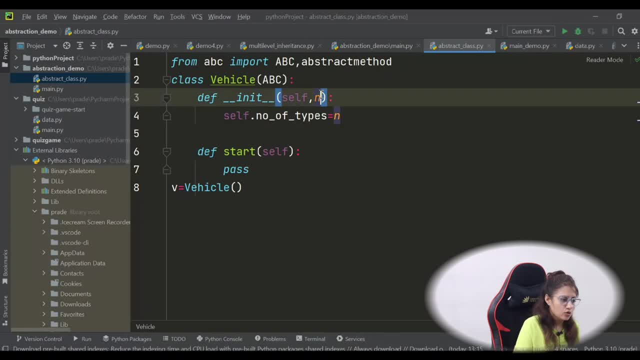 error type: error missing one required positional argument. so you have to pass here n number of tires, like suppose two. let's run this. see there is no error. so you are able to create abstract the method. you can say object of abstract class, because this is not abstract class. 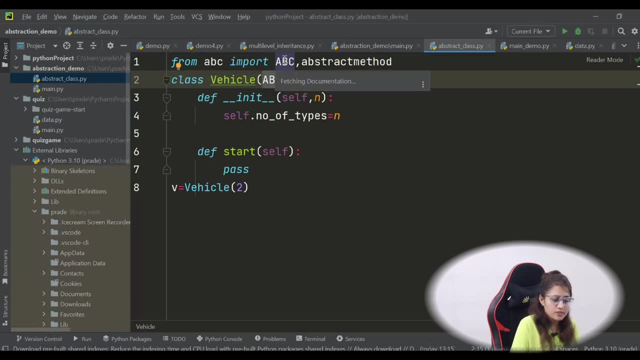 although you have inherited this class from abc, right then you can create object of abstract class. so let's you go through alone. we have done bu, but there is no abstract method. at least one method that is from abc module, abstract-based classes module, but still there is no abstract method. 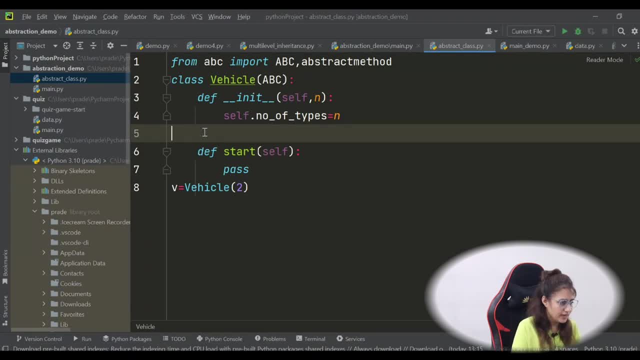 that is why it is not an abstract class. so you have to make at least one method abstract. now this class is a perfect class. right, then can be now. second point is what. there can be normal method as well in the substrate class, or you can say concrete method. 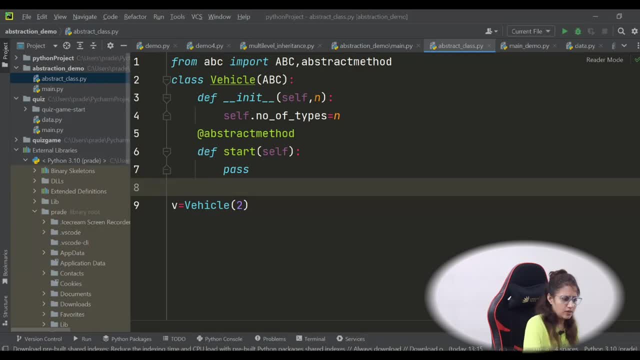 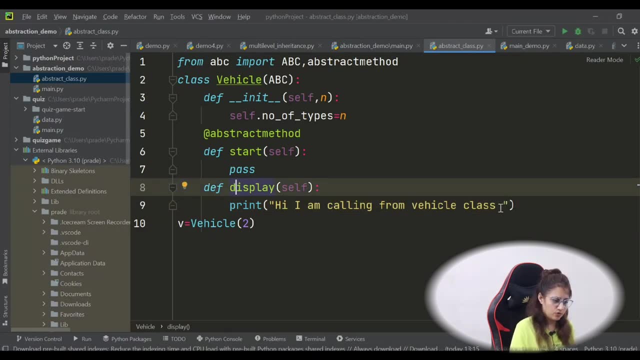 means normal method means they are having their definition right. so if i define a function here, like maybe a method, we are having display and hi, I am calling from vehicle class. any method you can have, we have display method. so one method is abstract method and one method we have. 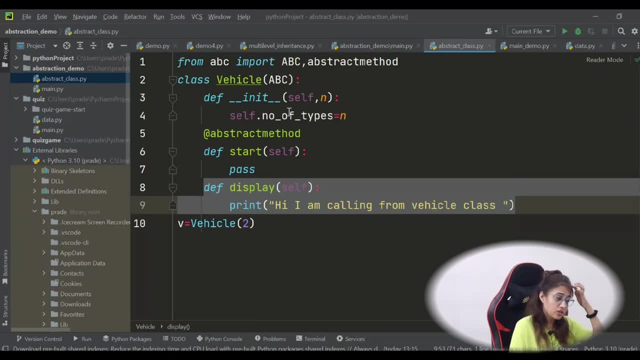 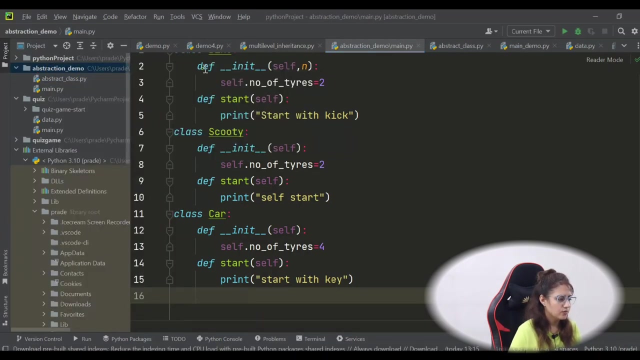 concrete method, any normal method. so our abstract class can have both abstract method as well as concrete method, or you can say normal method, those method which are having implementation. those are concrete methods. right, and suppose I am having one more file and the name of that file is main dot py. okay, we have already have main dot py, so main underscore, abstract dot py. 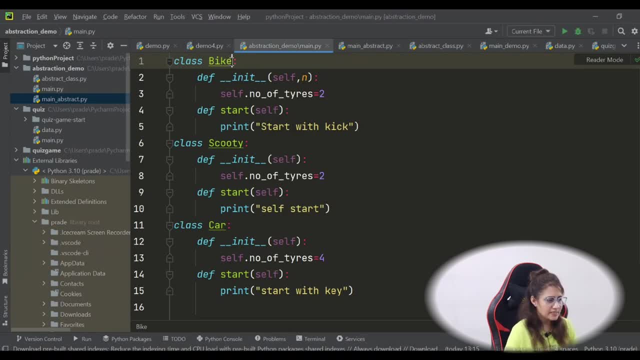 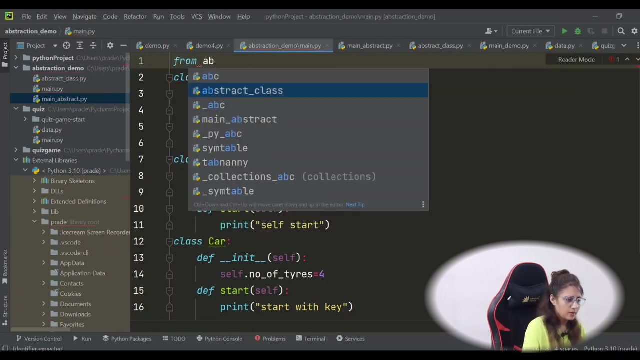 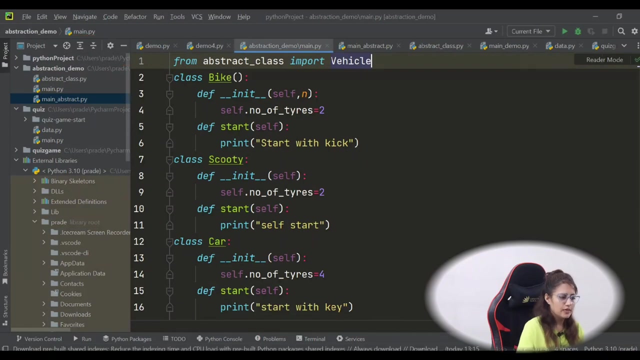 now, okay, first of all we are going to inherit these classes from our vehicle class, right, but see, there is, there is a, there is a, there is no. you can say that vehicle class here, see value error and overflow. that is it. so first of all you have to import vehicle class. so from the class name is from abstract underscore class, you have to import vehicle class, right, and then here now see classes, vehicle class from abstract class, this thing. so 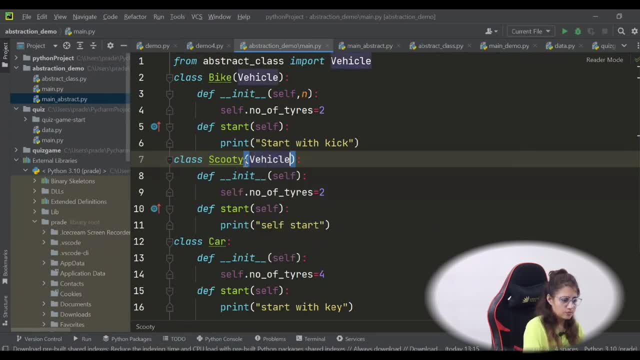 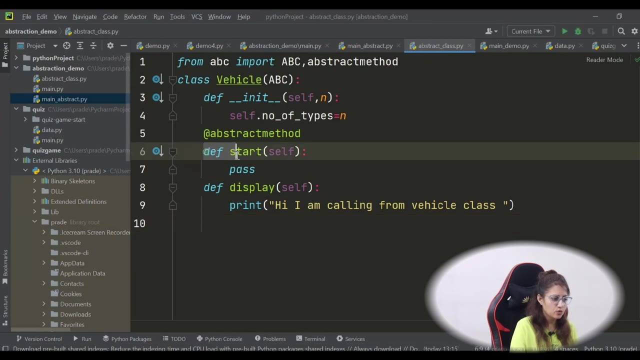 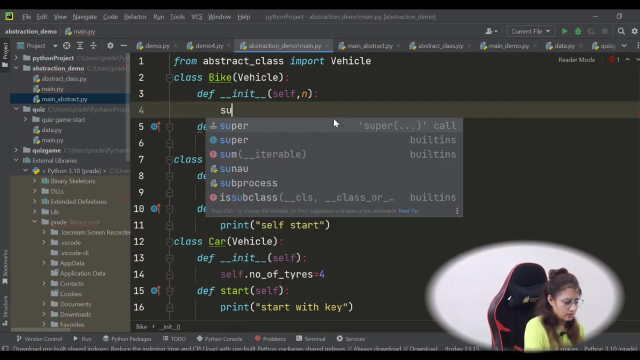 we are going to import these, all these classes, from vehicle class, right, okay, now they are having their own definition of this start function by every class and abstract abstract class. we don't have any implementation, right? so, rather than this, we can do what we can call this one super doh. 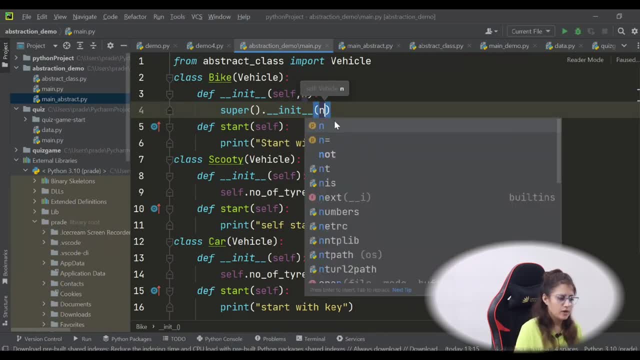 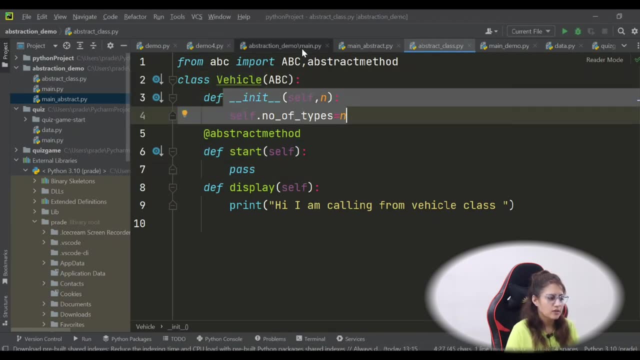 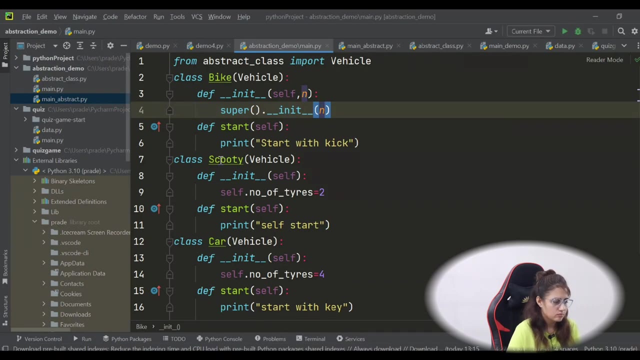 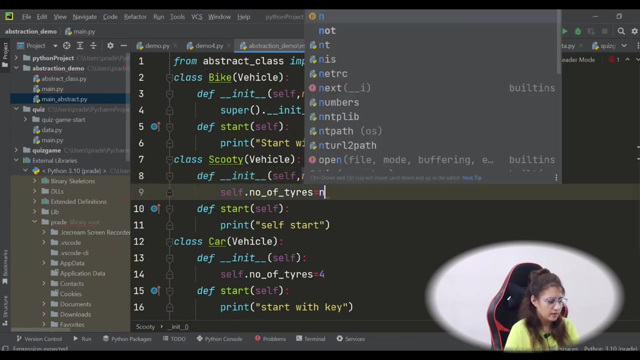 int and just pass n one parameter, because in super class is vehicle class there are, we are having constructor, so we can just call this constructor here super dot int, right? or you don't want to call? then simply you can write down here like comma n and is equal to n. you can define your own init on. 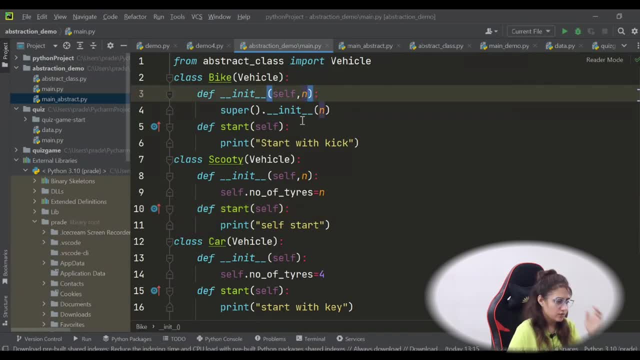 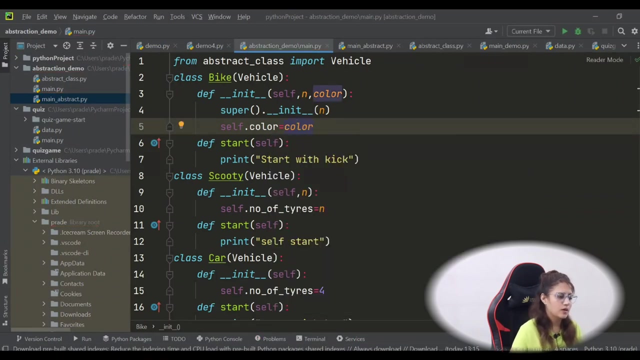 constructor. right, like one more thing. i want to specify here number of tire as well. as i want to specify for my bike class some other attribute you can also add right, like number of tire as well. as i want to pass color self to color is equal to color. that is also fine, so same for these we can. 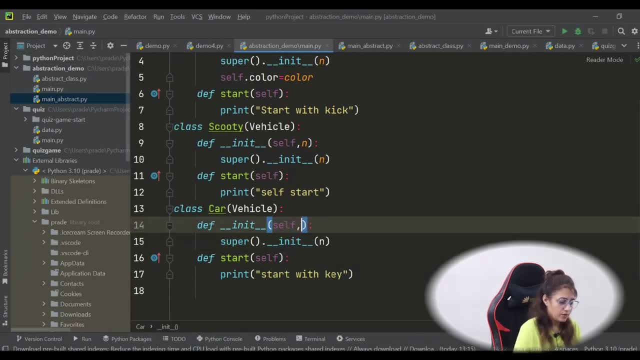 call unit constructor of super class, like in car. if i want to specify n as well as i want to specify like number of gears, right, let's take a parameter x and let's take self dot number of gears as equal to how many gears? five or six, five and one is back here, so let's suppose total six number. 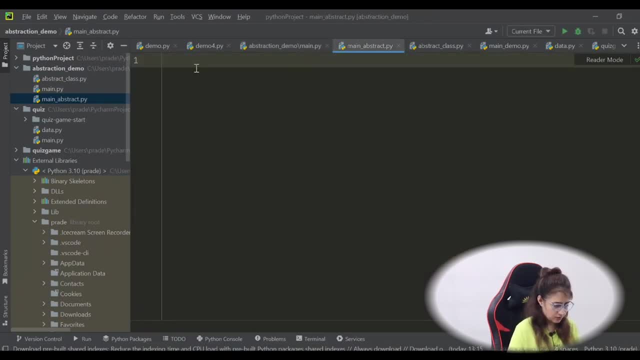 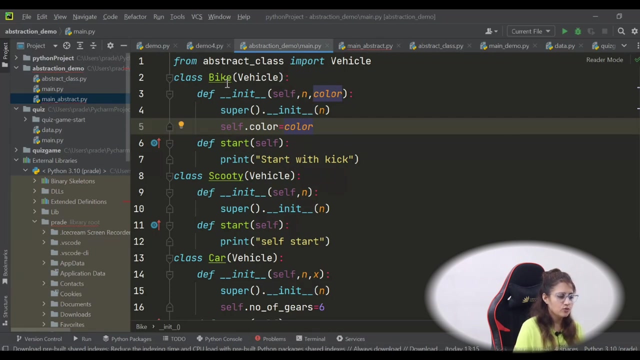 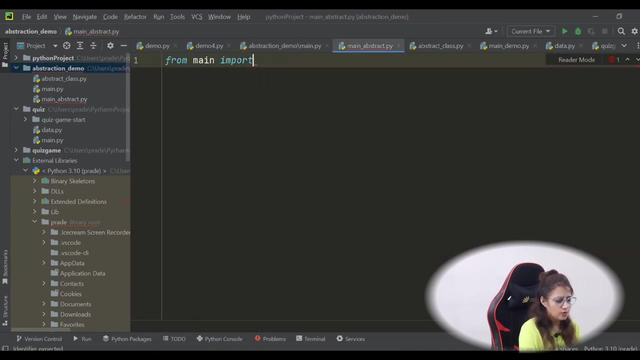 of gears. number of gears: six right in main class. we are going to create object of these classes and we are going to call start start function. so from abstraction demo from this class you have to import first all the classes, bikes, putty, and from main we are going to import. 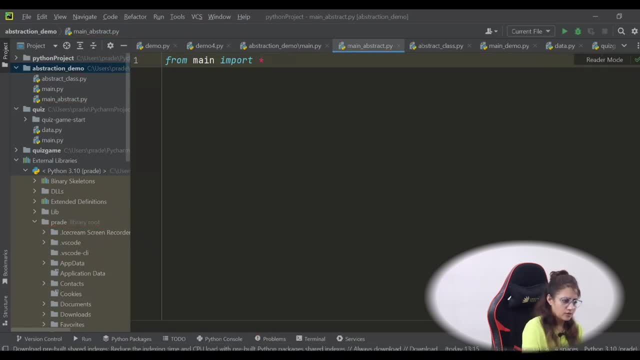 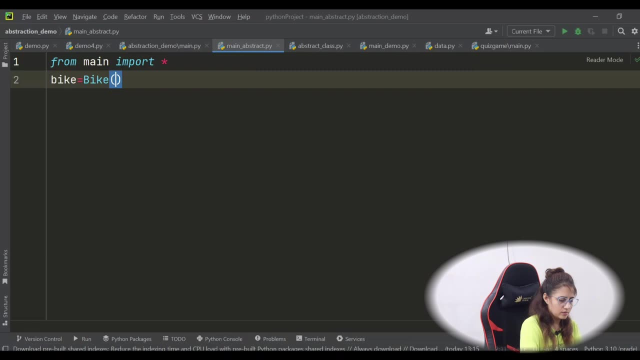 all the classes, so it's start. now create object of, suppose bike class, and you have to pass to one parameter, that is number of tires and c. you can see n and color, so let's pass the color, as maybe like black right, and using this object bike, we are going to call start, so let's run this one. 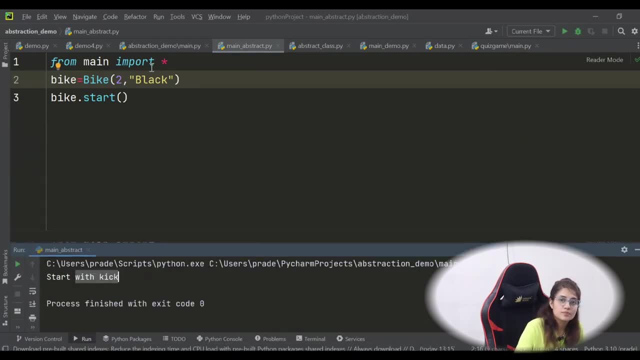 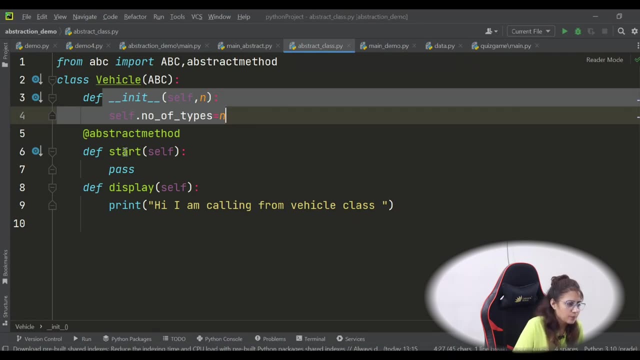 and see: start with kick right. so now see, if you look at this abstract class, then the methods are having no implementation means, basically, we are hiding, we are just showing the functionality, like obviously every vehicle is going to start, but we are hiding how it is going to start, right, and every class, every class which? 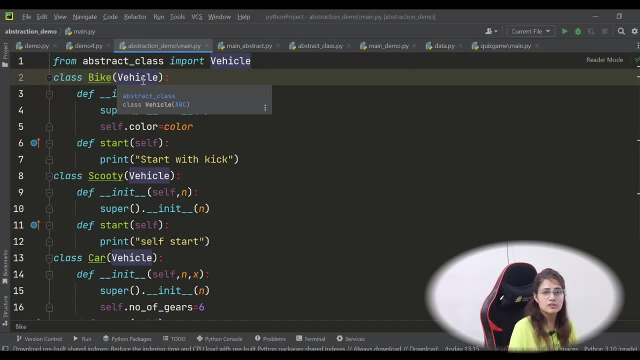 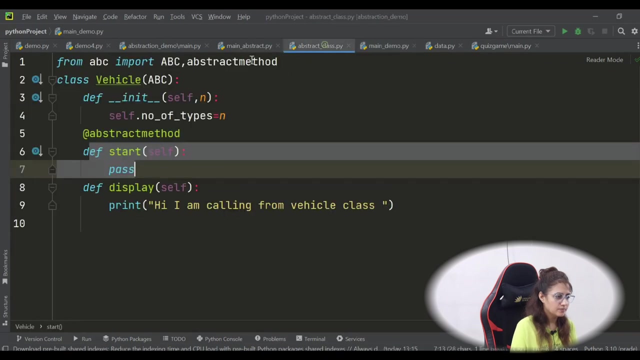 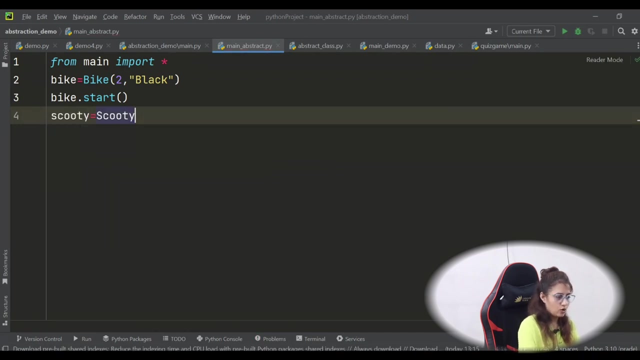 which is inheriting this vehicle class, give their own implementation of the subtract method. and it is compulsory for every subclass of vehicle class to implement the abstract method. if suppose in scooty I don't implement this start method right, so now let's create in main, in main class, let's create object of. 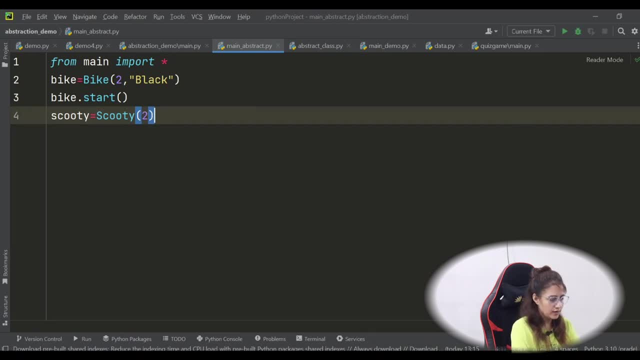 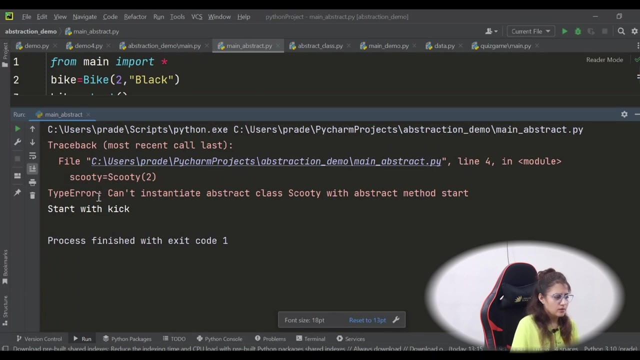 scooty right and scooty, let's pass number of tires to and with the help of object, I want to call start. so you are not able to create like object of this scooty. let's run this: see. cannot instantiate abstract class scooty with abstract method start: see. 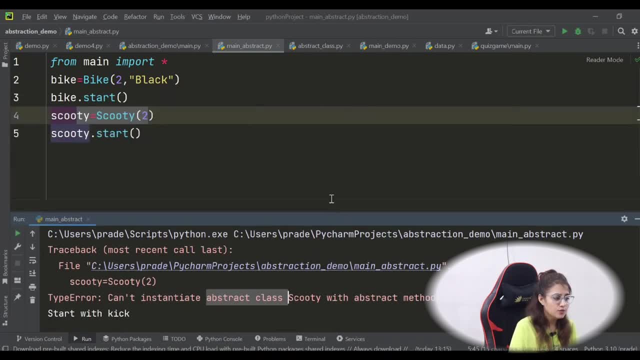 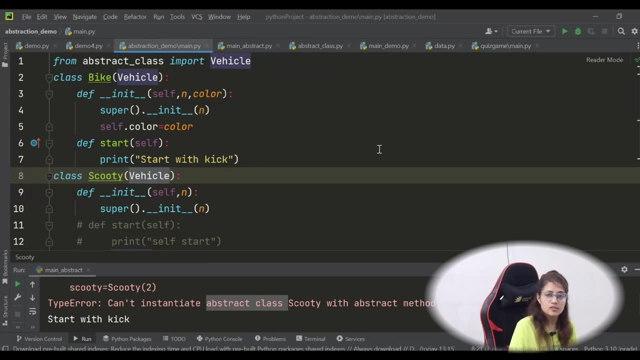 scooty is now abstract class. so if you are importing, if you are inheriting a class from an abstract class, then two choices you have: either you have to implement all the abstract methods right, otherwise make the subclass as an abstract class. now scooty is also an abstract class. 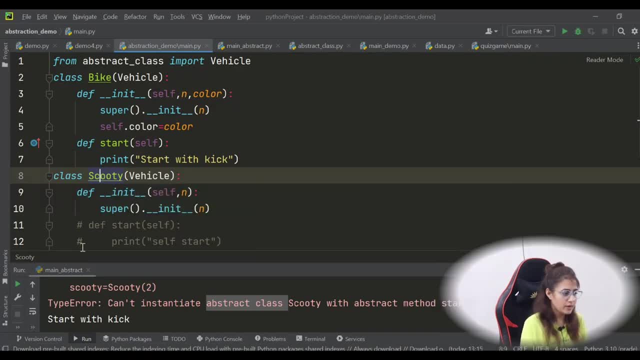 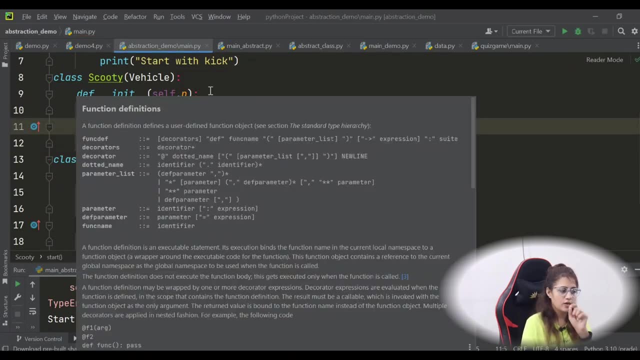 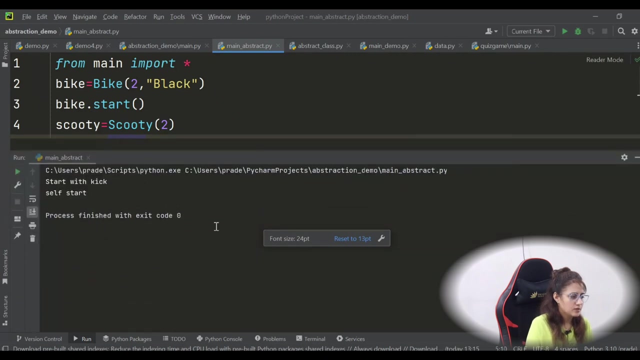 okay, it's fine. but if you want that, scooty should not be an abstract class, you have to define, you have to define the abstract method here right now it will run. let's run this see: start with kick and self start for scooty self start. 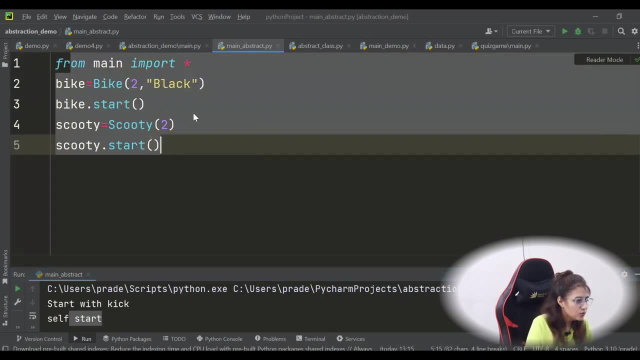 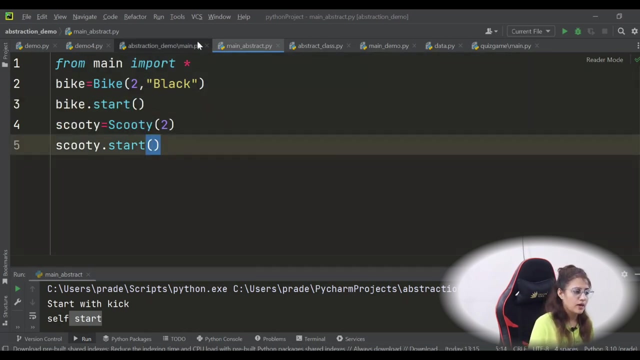 right. so now in this, see, we are just, we are just calling the method start and right. we don't know the implementation of start method and we don't need to know the implementation of start method, right for bike and for scooty, you just need to know the function name or maybe, if any parameter to be passed, and that. 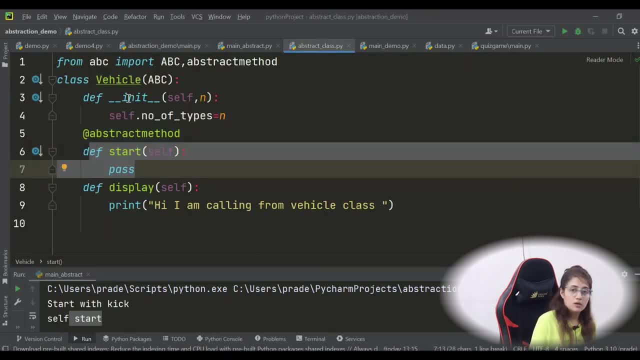 obviously we can. you know we can see from the substrate class, right? so implementation we are hiding, we are just showing the functionality, that is, start. there is no implementation of the start method, so we are just showing the information. so we are hiding basically the implementation detail, that is. 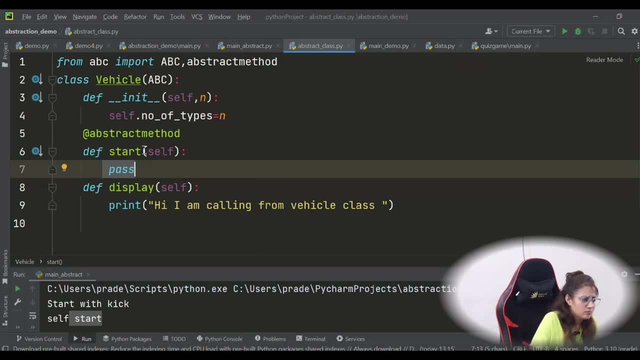 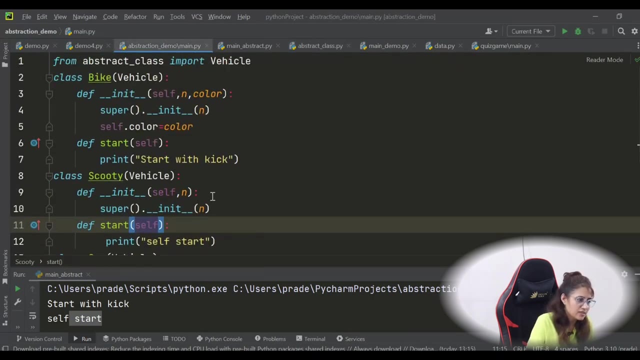 abstraction right now. why we are creating this. you know upset class and we are just defining an abstract method here: start because we don't need to create pickle class and directly we can create these classes and start with kick and define the start method in these classes. so what is need of the substrate? 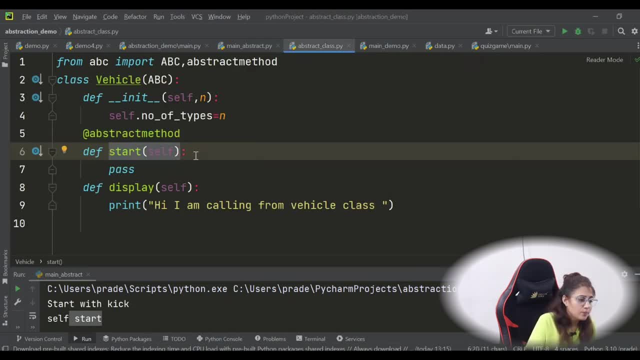 class right. okay, the principal point is that we are hiding. basically, the problem is: see, if you want, if you are working on a project which are having many classes and every class is having same method, like here, start method right. so if you don't define any rule, then 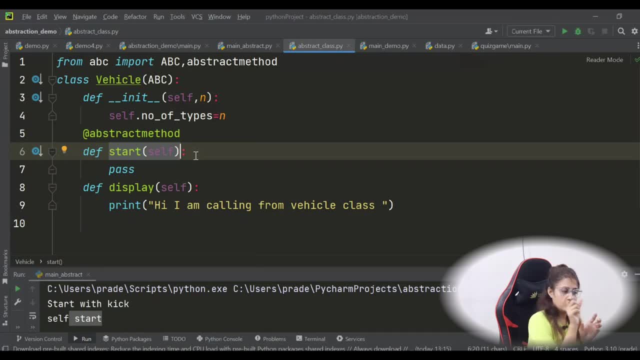 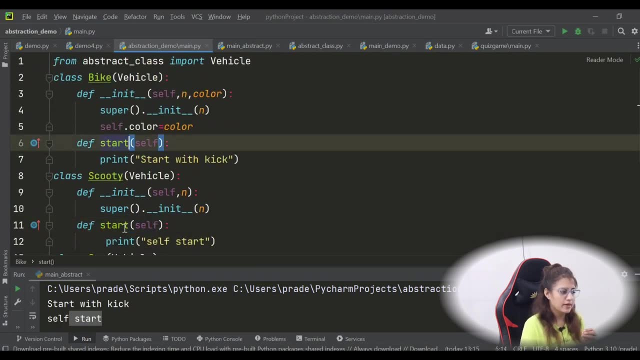 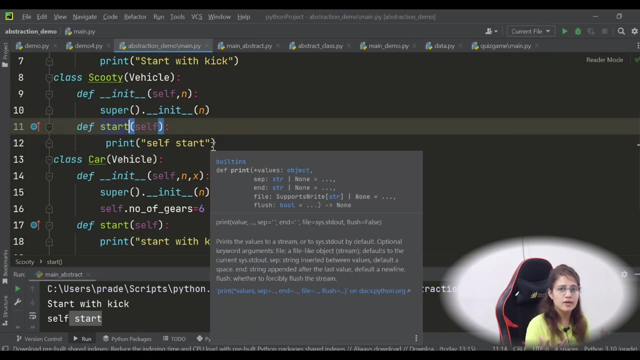 every class maybe define their own name of that method, like start underscore, maybe like in bike. in this i'm going to define this method: start underscore bike, or start underscore s or car underscore start. so every class is defining that method, having their own name, and like this: 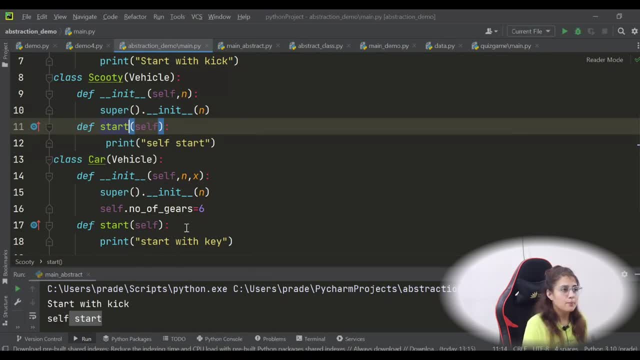 number of parameter, their own parameter, right, but obviously method is same start. so it's better to enforce some structure, some rules, some blueprint, right, like every class is having this method. the name is this and every class is going to implement this method. okay, if you want to use my vehicle class, if you want to make a subclass from my vehicle class, right. 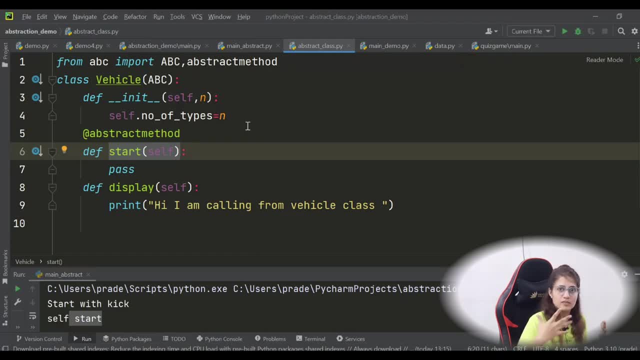 so if you want to define some rule, like if you want to come in my class, there are some rules: you have to be on time, right. and second thing, you have to come with at least one notebook and one pen, right? these are some rules. so i have defined rules, some for my, for my class, right. 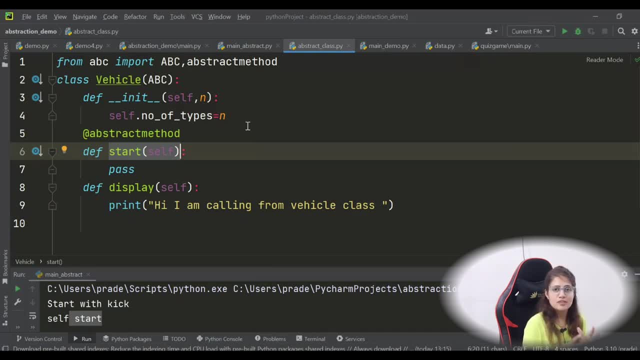 so like this: also, we can define some specific rules. every subclass has to follow those rules and it's completely fine to not use upset classes and abstract method without this. also, we can, you can, we can, uh, you know, implement, we can, uh, create our project or we can write down our program. but when we are dealing with large software, large project, 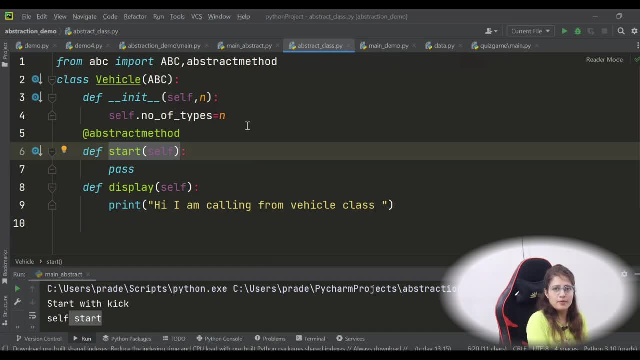 in that case it is compulsory, like it's a requirement, basically to implement abstract classes, to implement abstraction, to use abstract methods, and all right. so maybe, if you are not you know getting the use of this thing, it's fine, you just have to be. you just have some idea. you have to be clear, like: what is abstract class? 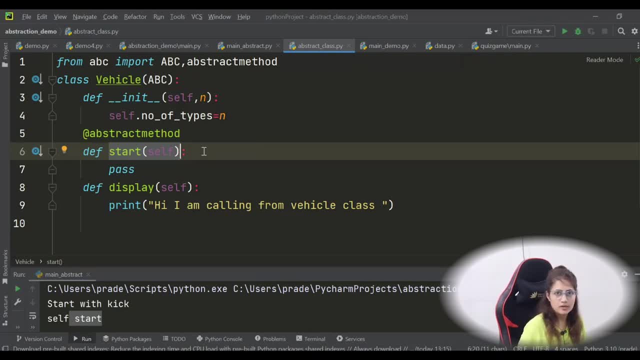 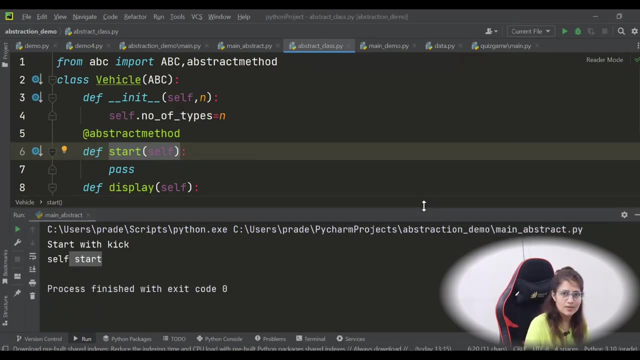 what is abstract method, the rules, and all right, maybe when you are, when you will be working on a project, then definitely, when you will use this in real time, right, then definitely you will get the use of this thing. fine, so, like here, it's true. so, rudy whites, here is url and rule number three. 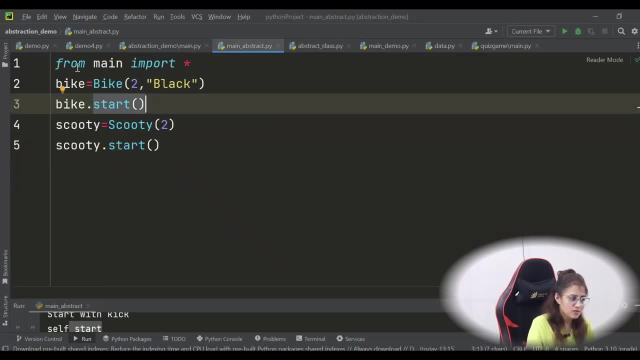 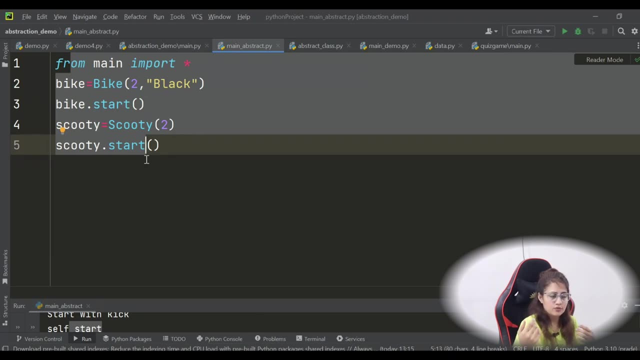 we don't know the implementation of the start method, but we are getting the result right from this main file only right like this. also, we use many like if you are working on list. there are many inbuilt functions like reverse a list, sort a list right, append that we discussed like 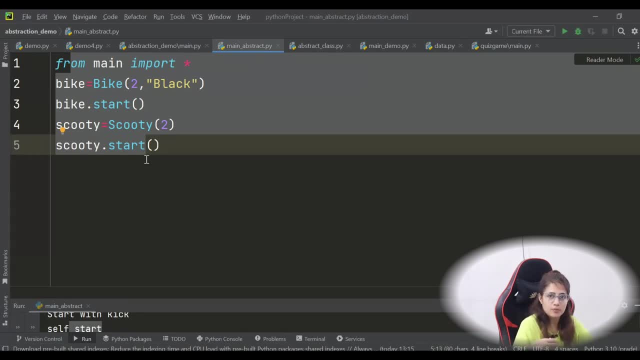 random function. also, we have to generate a random number. fine, so you just, if you are having a list, you just use that function, like maybe you are using a reverse and it will, it is going to reverse the list. you don't know the implementation, how it is going to reverse the list, right, so that? 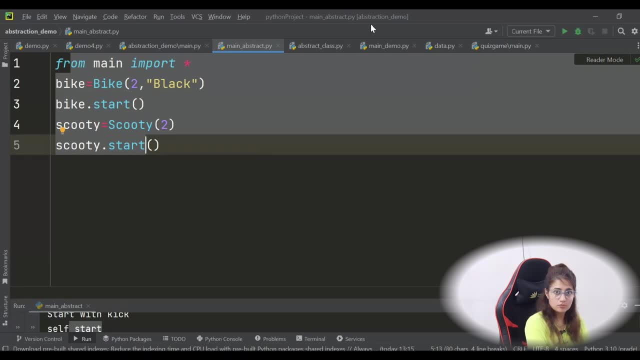 implementation is hidden from you. so that is beauty of abstraction. okay, so it is going to make the life of other developers easy. you can use those inbuilt functions also. also right, so that is, you can say it's a type of abstraction, only fine. so in brief, if i say what is abstract class? a class having one or more abstract method is: 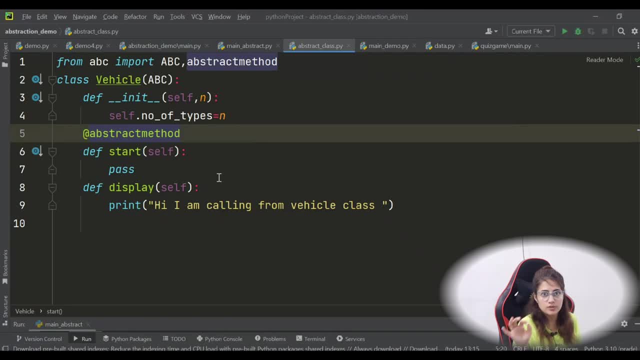 known as abstract class. and abstract class cannot be instantiated. no object can be created from abstract class, right, an abstract class can have abstract method as well as normal method. or you can say concrete method. right, we can say like a class derived from abc class which belongs to 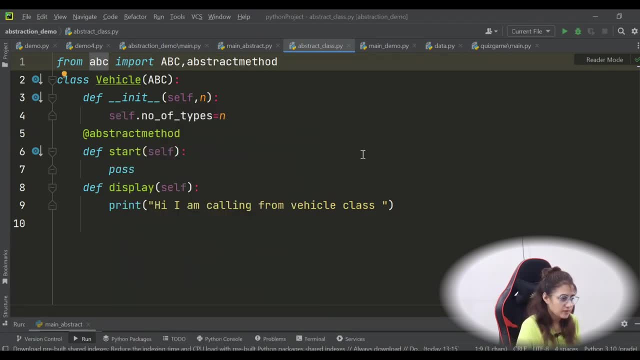 abc module is known as abstract class right. and what is abstract method? a method which has only declaration, no implementation. that is abstract method right. you have to use a decorator at that abstract method to make a method abstract method right and abstract method in a base class. obviously this vehicle is like a base class. every other class is subclass of vehicle class right. 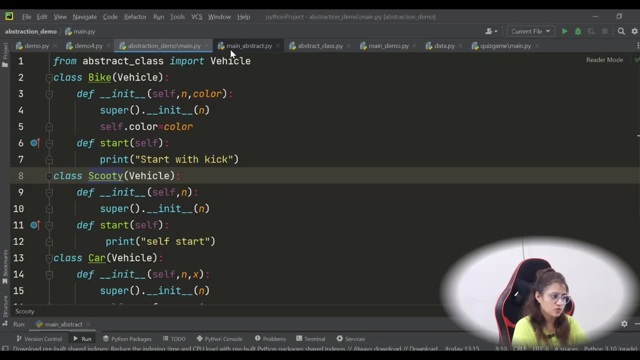 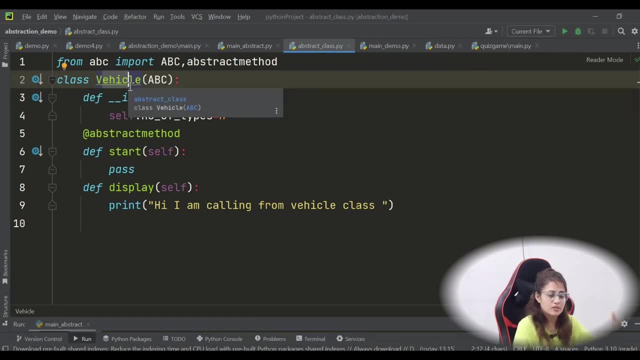 like this: by x to t. these are subclasses of vehicle class. so this you can say abstract method in the base classes, just show the functionality. see it is showing the functionality. start right. but many functionalities we can show, many abstract method we can use. just show the functionalities and those functionalities should. 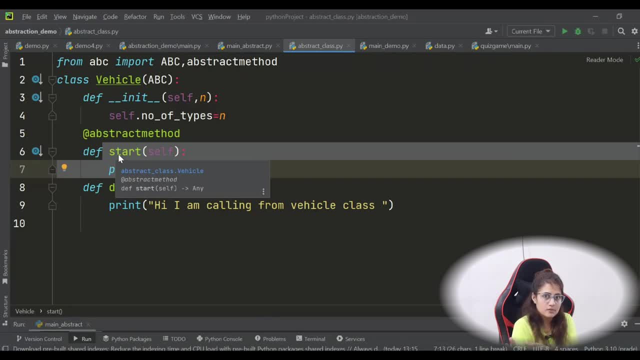 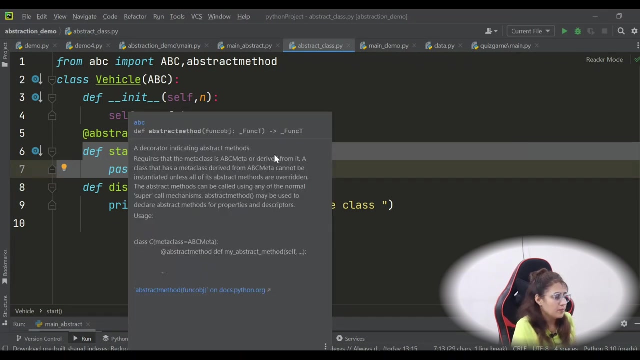 be implemented by the subclasses. right, if any other class wants to use my vehicle class, then that class must have to implement this start method. otherwise that subclass also we will be considered as abstract class. right, so the subclasses can have implementation of the abstract method according to their 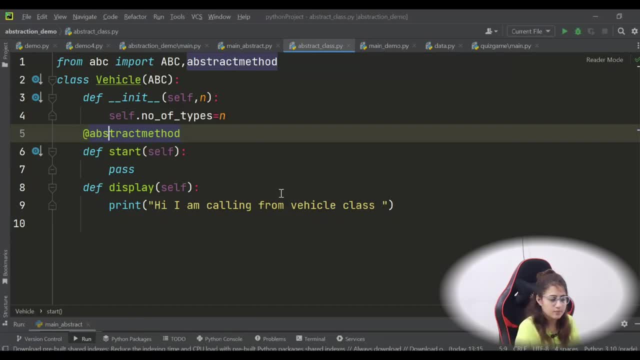 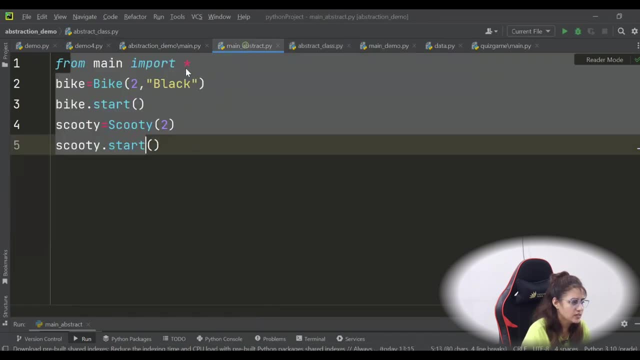 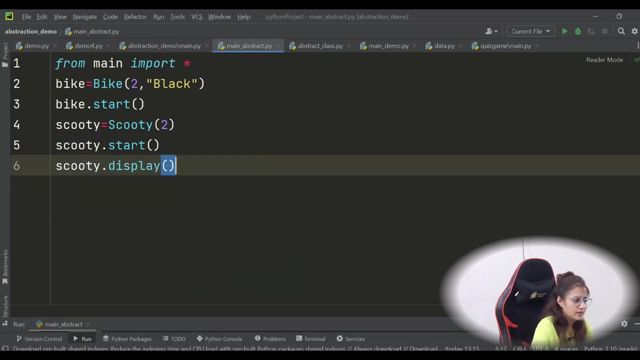 need. every subclass can have its own implementation. right and see, this display is not an abstract method. so if you want to call, if you want to access this display also, then also we can do with the help of like scuti objects, scuti dot display. so it will run and it will, i am. 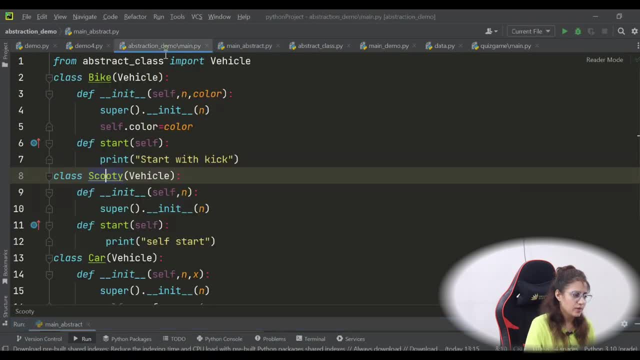 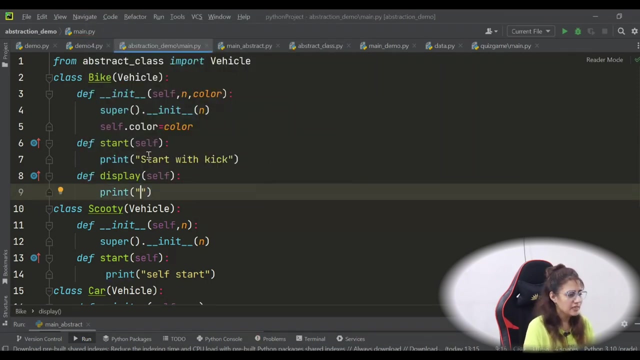 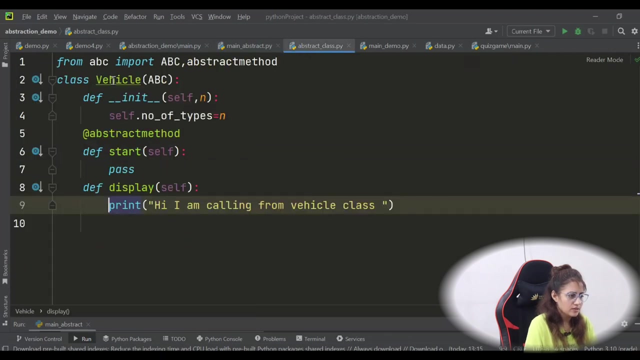 calling from vehicle class right. we are calling from the vehicle class right and it will run calling this display of this class, abstract class using scutty object or see, if you want to override see. this is basically what nothing but method overriding means in this class in base. 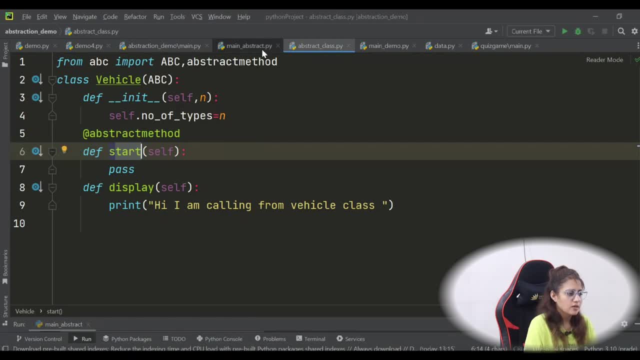 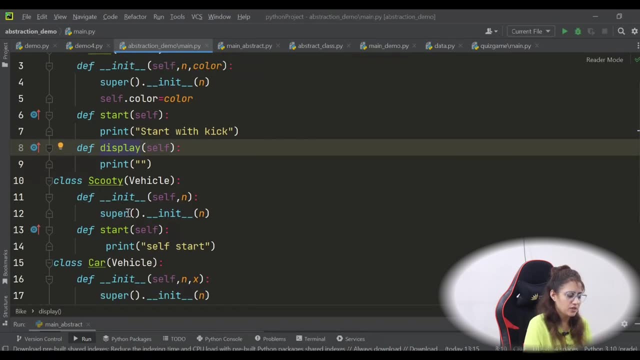 class. this vehicle is base class. we are having a method start and we are just overriding this method according to our requirement in the sub classes. right overriding means we are giving our own definition of this method right. so same for display. also, like i want to print the color of 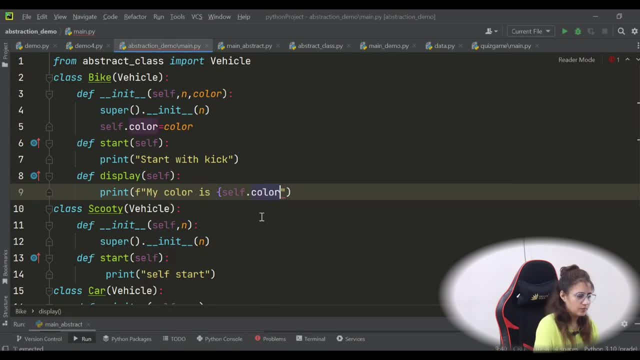 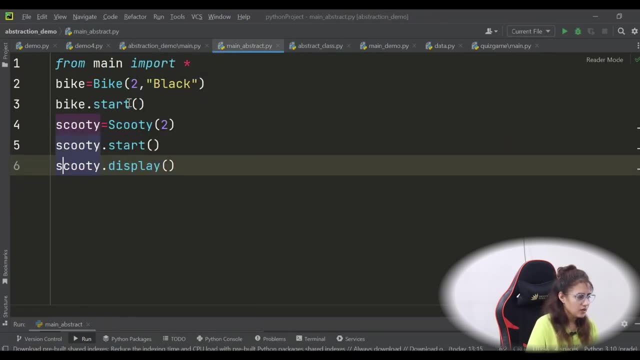 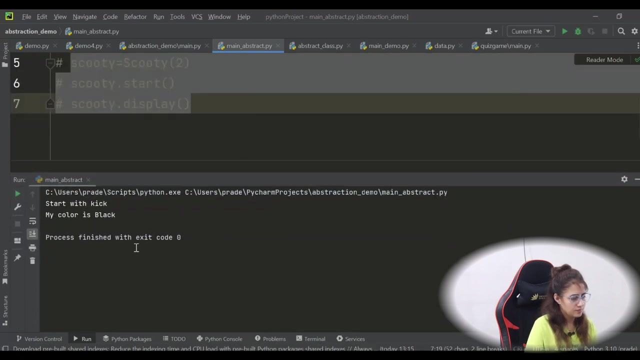 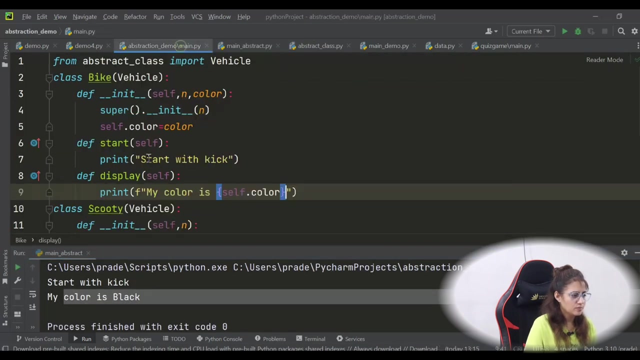 the bike. so dot, self dot color right and with the help of uh bike, now just call display. now let's comment this out and let's run this. see, now start with the kick and my color is black. so this display we are calling from this one. my color is self dot color black because we